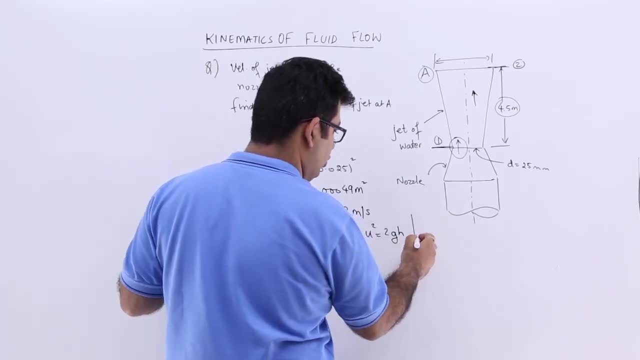 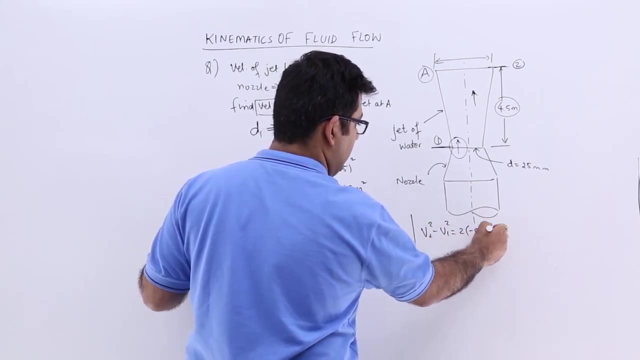 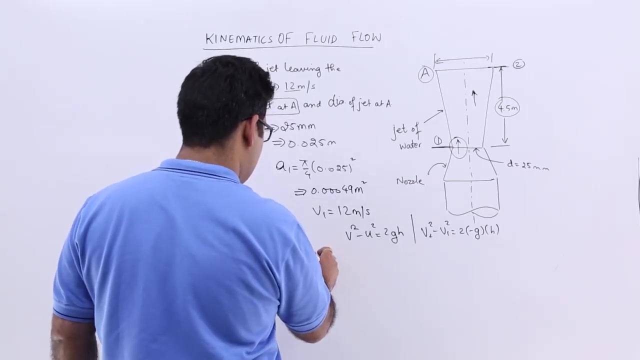 So V is the final velocity, that is V2.. So V2 square minus V1 square is equal to 2 into minus g, into h. From here I can easily find the value for V2.. So V2 would be under root V1 square. 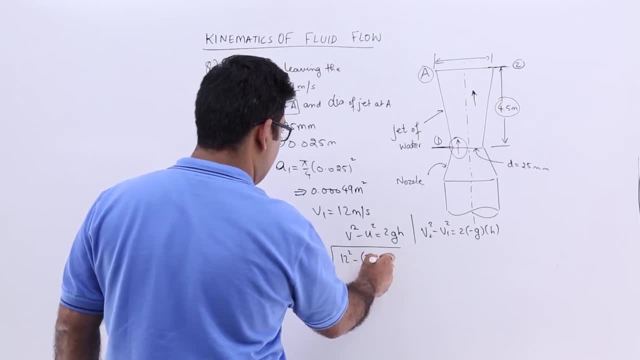 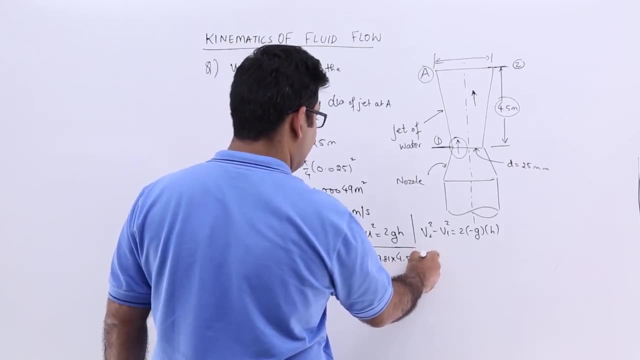 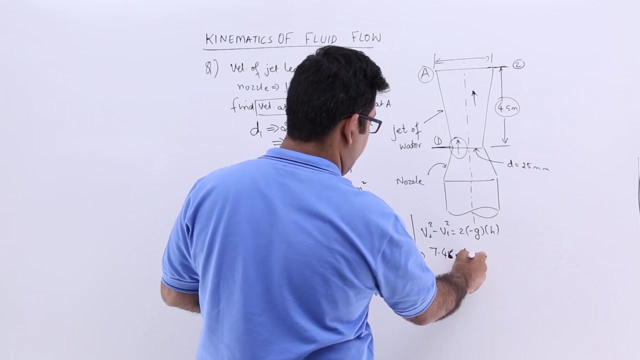 V1 square, which is 12 square minus 2, into 9.81. into h, h is 4.5 and this will give us a value of V2 as approximately 7.5 or, to be exact, I will write down 7.46 meters per second. 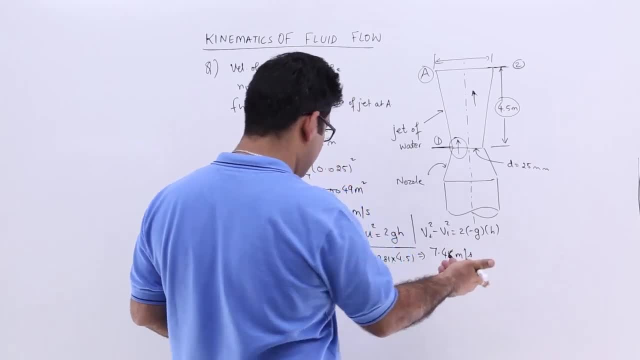 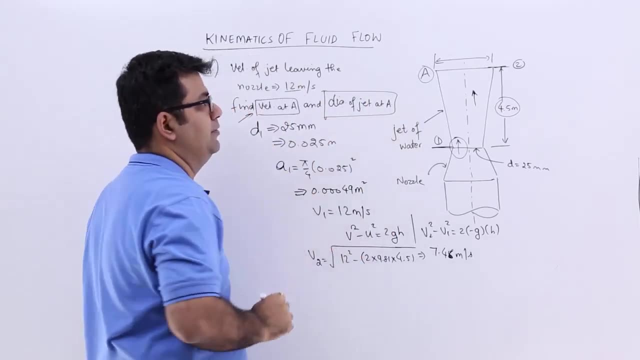 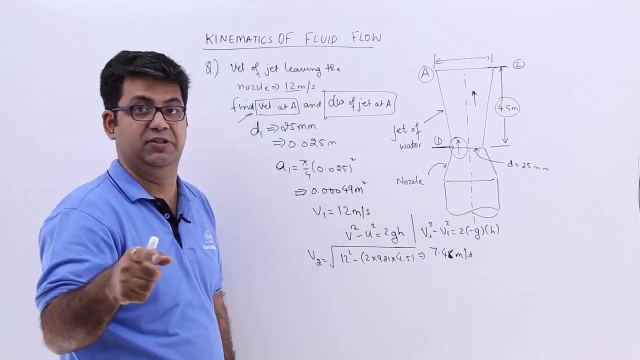 Okay, Now I have got the value for V2. that is this part. Now we need to find the dia of the jet, Of the jet at section A or point A. Okay, So how do you find the dia? So you need to find the area first. 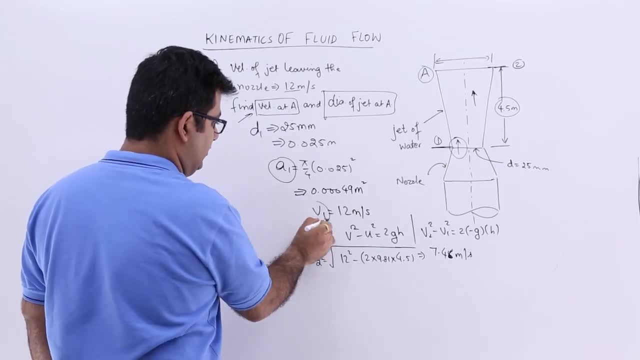 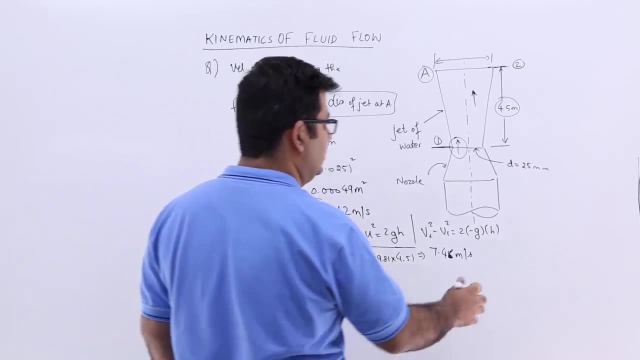 Okay, So area. So we have area 1. We have velocity 1. We have velocity 2. We can find out area 2 by applying the continuity equation. So I can do this, That is, A2 into V2 is equal to A1 into V1.. 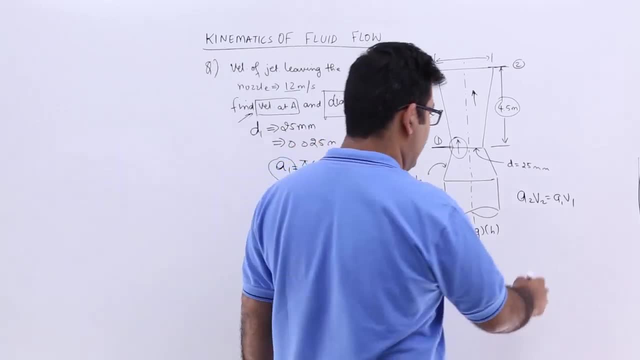 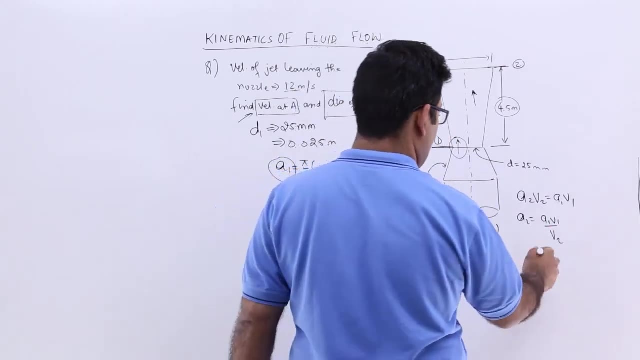 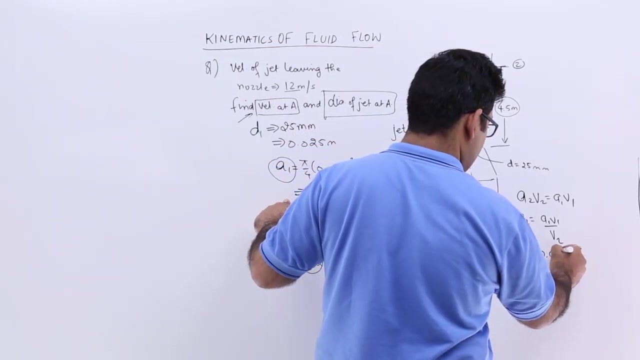 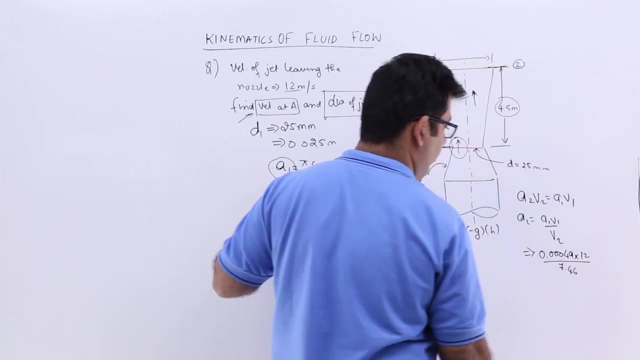 That is the continuity equation. So from here let us find out A2.. Which is A1, V1 upon V2.. So A1 is how much? A1 is 0.00049.. Okay, V1 is 12 and V2 is 7.46.. 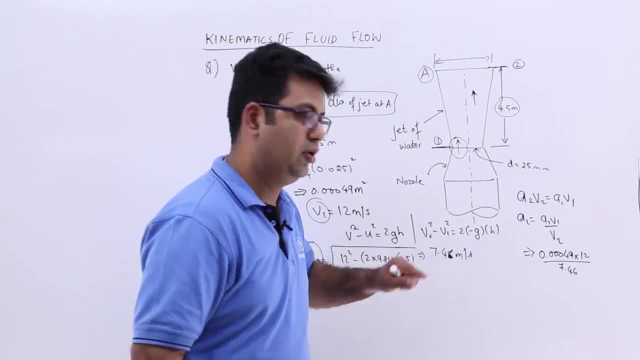 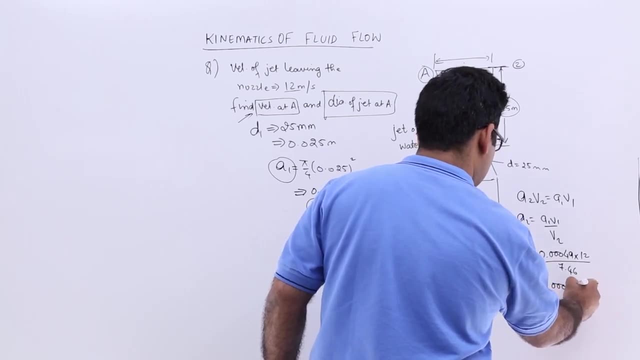 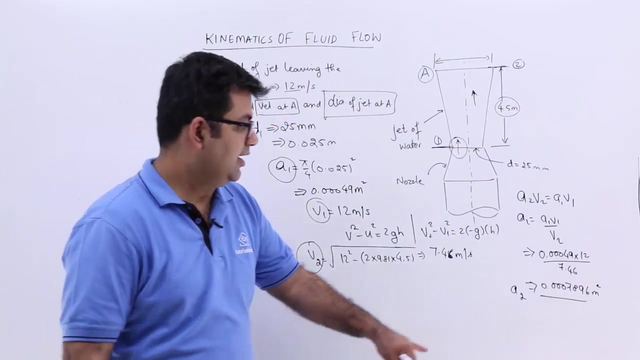 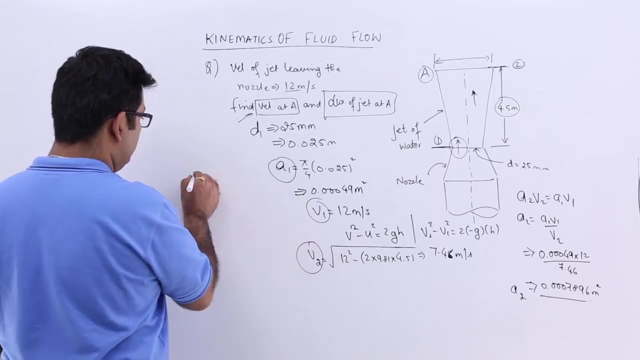 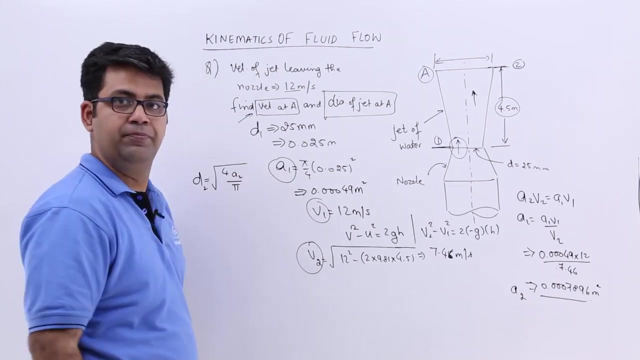 From here I can get the value for A2. So A2 would be 0.0007896 meter square And in relation to this A2 we can find out D2. So D2 is equal to 4 into A2 upon pi under root. 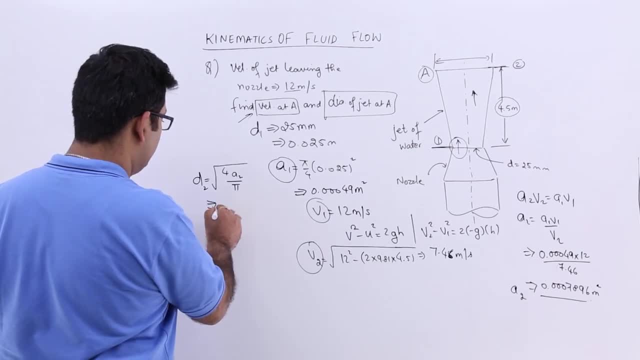 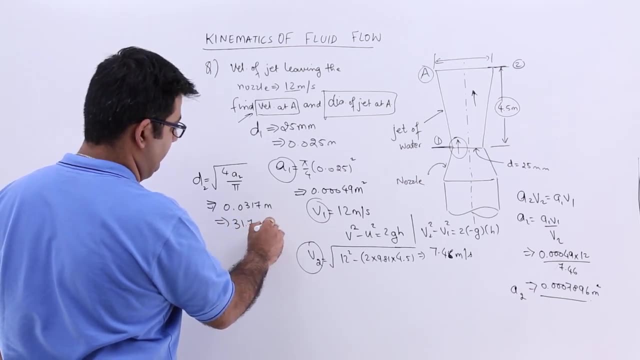 So when you put that value over here, The value of D2 comes out to be 0.0317 meter, Which is nothing but 31.7 millimeters. So this is the second part of the question. So it is a very simple question.